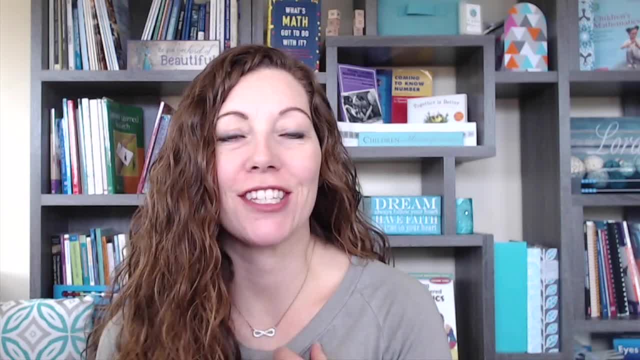 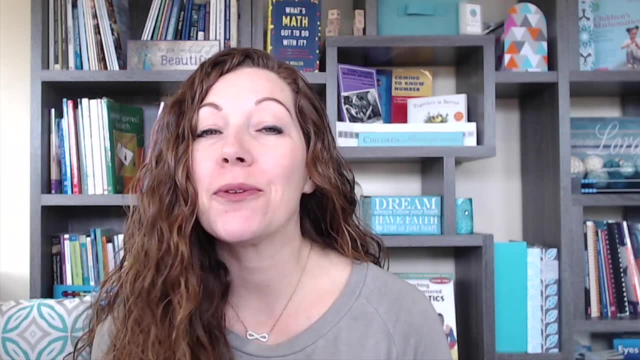 In a previous post, I gave you my recommendations of manipulatives that I love. Well, in today's video, I'm going to give you some rules when you are using manipulatives in your classroom. I'm Kristina Toneval, the Recovering Traditionalist, and today I'm going to give you 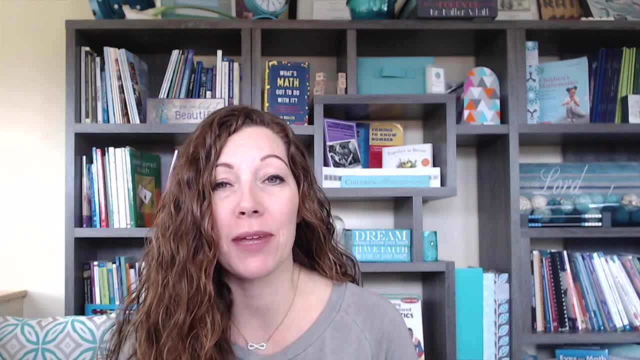 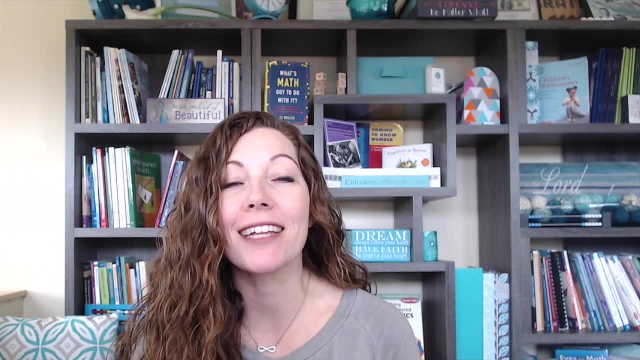 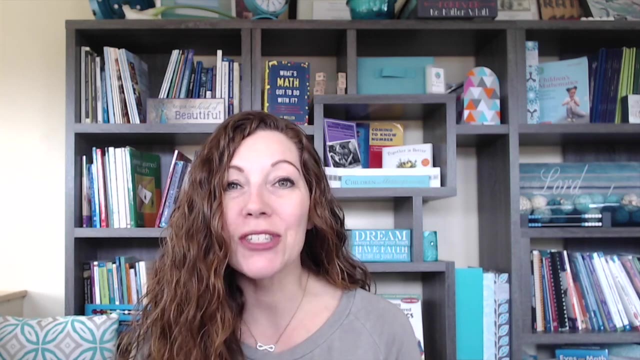 three rules for how to use math manipulatives in the elementary classroom in our quest to build our math minds, so we can build the math minds of our students. Okay, so rule number one is tied to the video I did before when I talked about my favorite math manipulatives, which is: 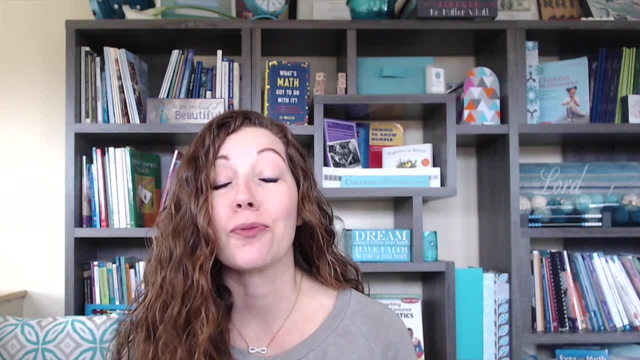 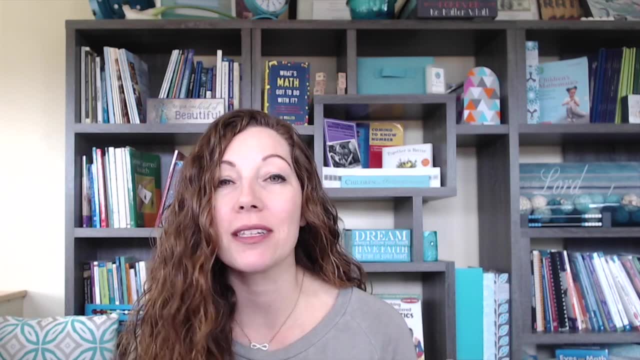 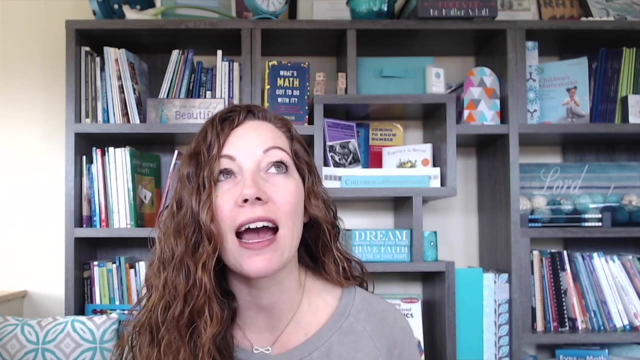 just to let the kids play. So rule number one: let the kids play. I'm not going to go too much in detail with this. I will link to the post below this video that talks more about that. but the general idea is that kids cannot develop an understanding of a manipulative and the 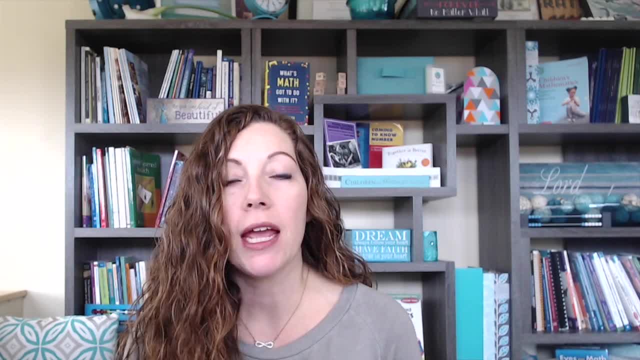 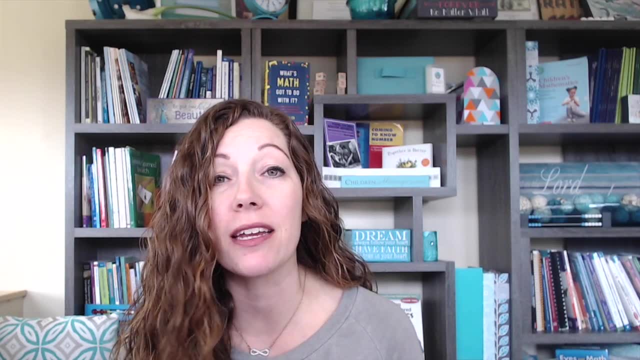 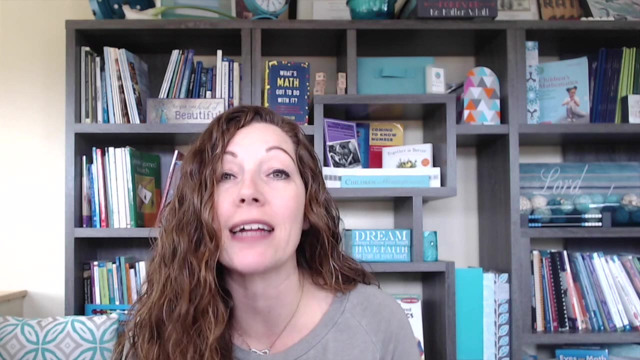 connections that that manipulative can build for them. if we try to directly teach them how to use the manipulative, They need to play and explore that manipulative and start to make connections on their own and we can help make those connections. but it doesn't come from directly. 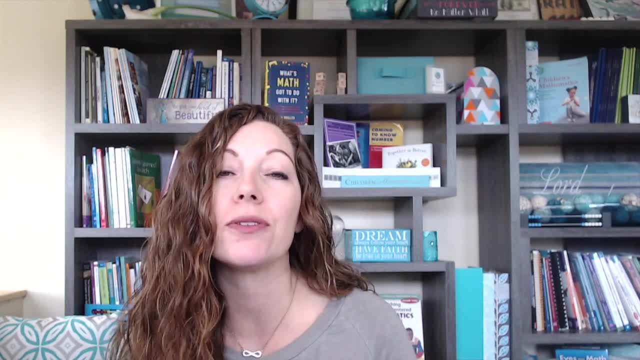 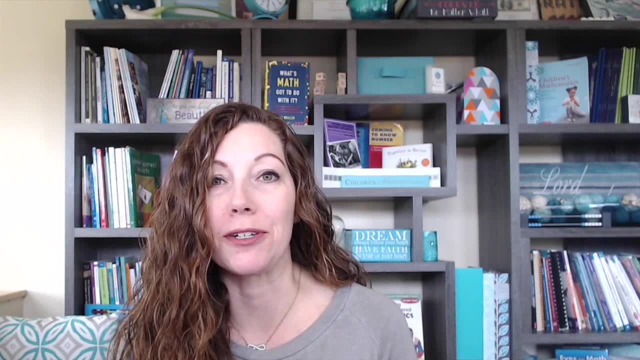 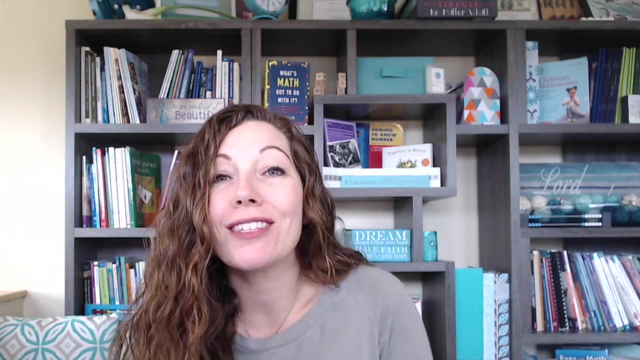 teaching kids step-by-step how to use a manipulative. Rule number two: always have manipulatives available. Typically, we just bring out the manipulatives when the lesson calls for it, So these are like special occasions, right for the. 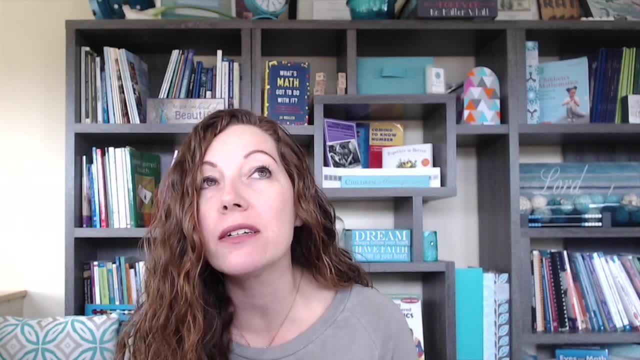 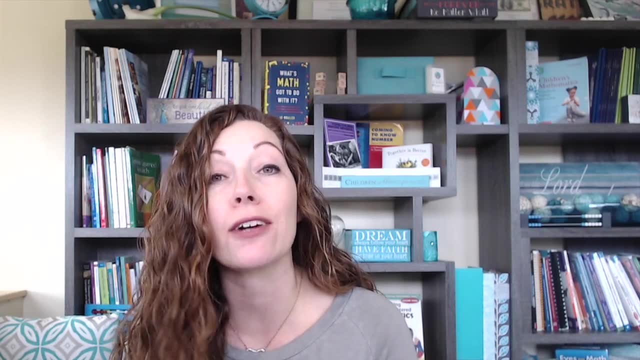 kids, and it's no wonder that we end up getting kids who will build swords out of unifix cubes. They're just not used to having the manipulatives as mathematical tools. If we have them out available all the time, then we're going to be able to use them. So rule number two: always have. 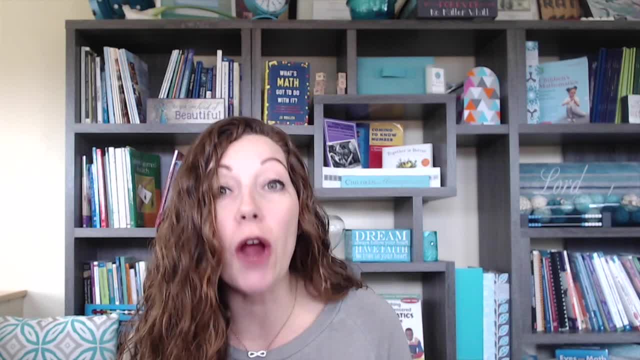 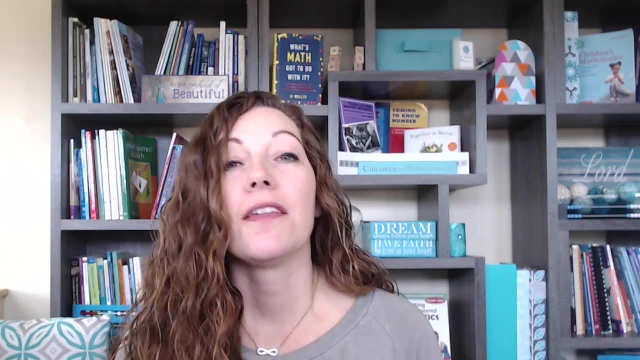 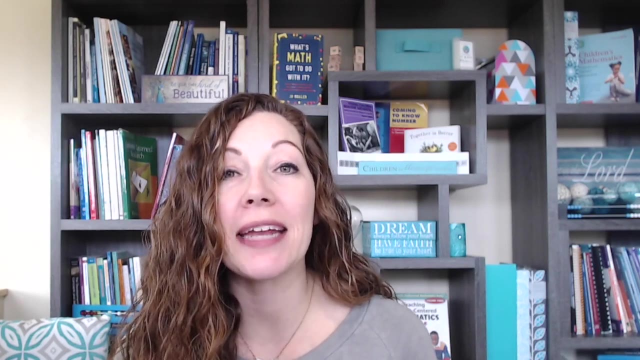 kids start to understand. these are mathematical tools. They are not toys that we only bring out and use on special occasions. There are lots of examples that you can find, especially out there on Pinterest and Instagram, of teachers who have created like a mathematical manipulative bar. 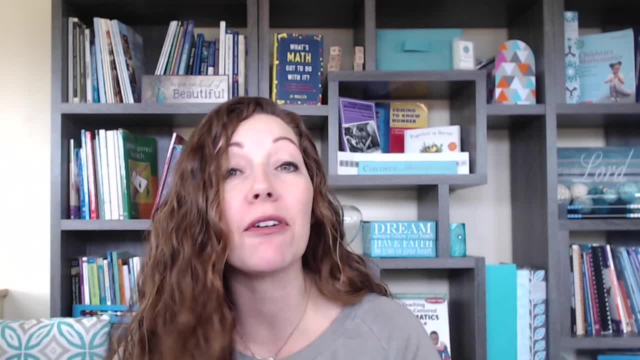 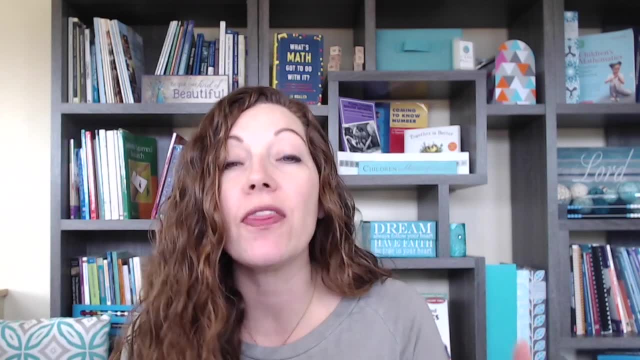 basically where they have it all laid out all the time and kids can come over and grab any manipulative they want. Or you'll see ones where they just have manipulative tubs that are on the tables right If you're in groups, in the center of those groups are 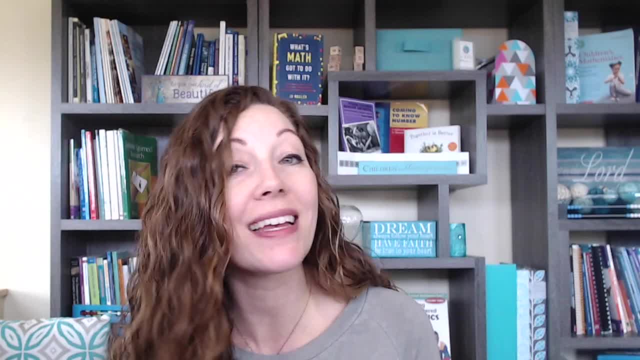 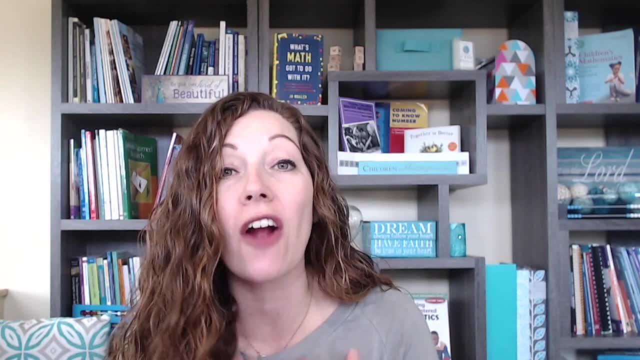 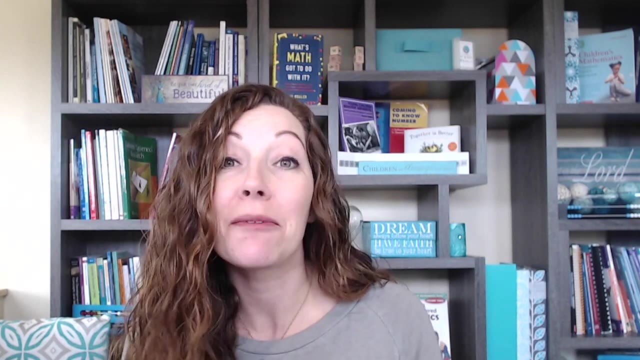 the manipulatives. They're always available so that if kids need them and want to use them to help them solve a problem, they can. We, as the teacher, are not dictating: here is the time to use the manipulative and here's the time when we don't. It's just: if you need them, let's use them. 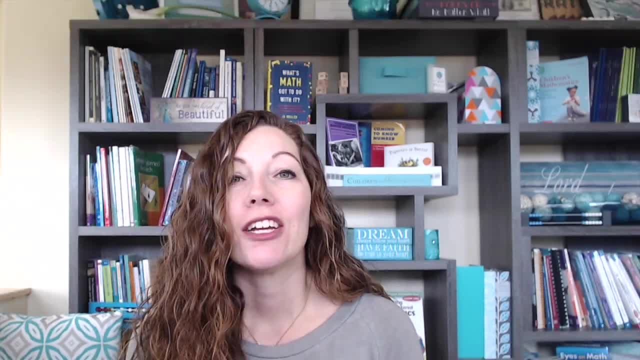 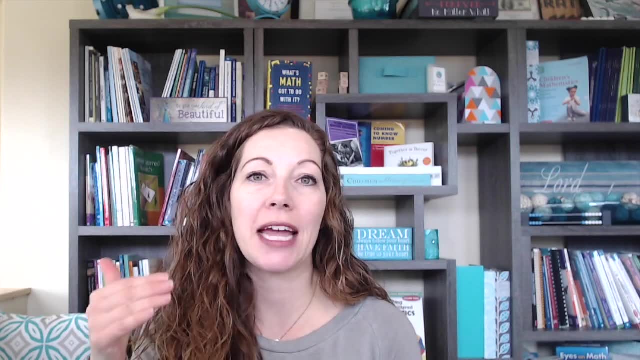 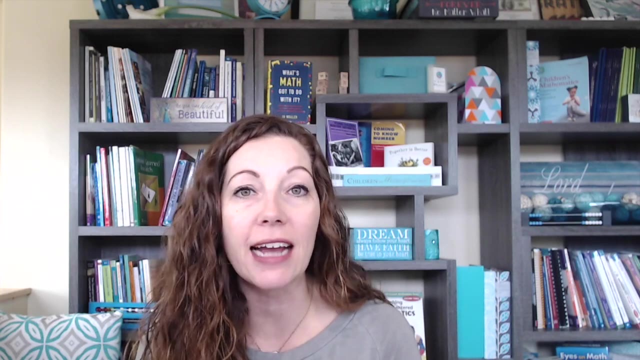 Okay now. rule number three: use manipulatives in isolation. So when we tend to do like a lesson and it says to use a manipulative, we tend to just use the manipulative and not connect it to those other parts of the CRA. 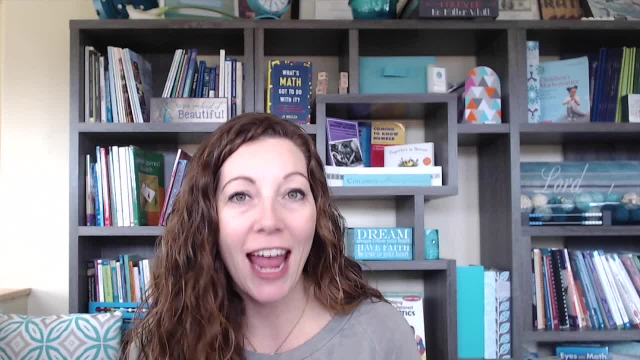 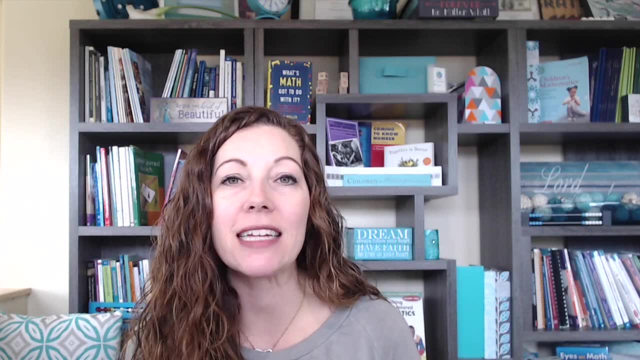 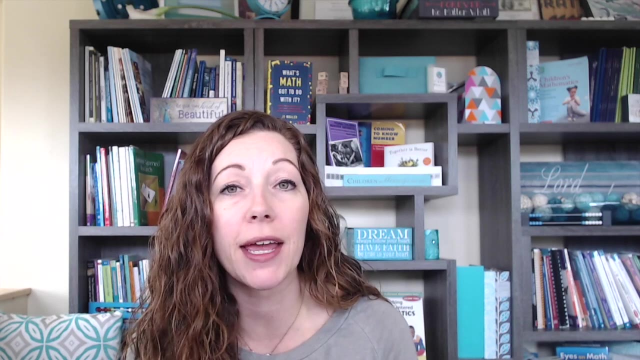 model. Now, if you're not familiar with CRA, I did another video all about that, which I will link below this. but the C stands for concrete, and that's typically the manipulatives. R stands for representation, which is often a model or a drawing, and A is abstract. 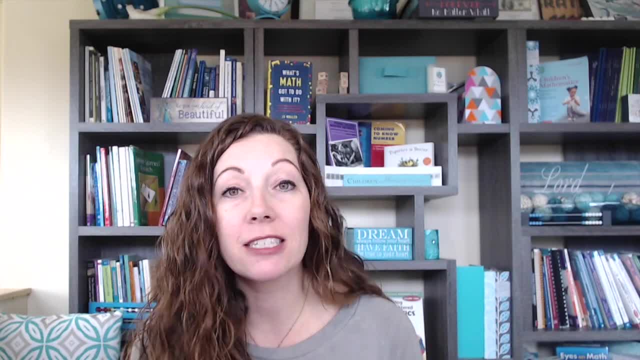 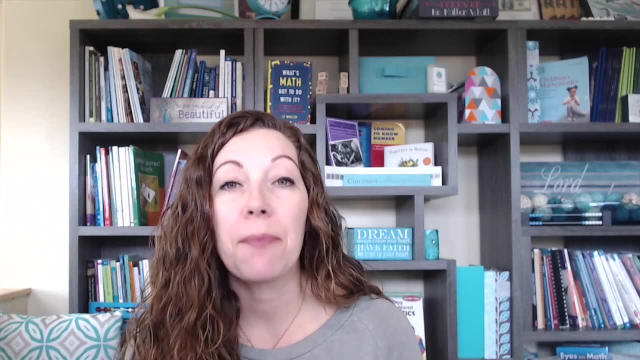 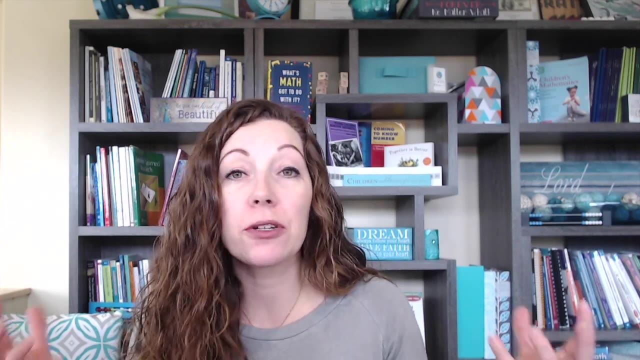 which is just the symbols. Our textbooks typically will have a lesson that is concrete, so it uses manipulatives. Instead, my advice is that we should be doing all three together as much as we can, and if the kids need it, Like we're doing a problem, and if some kids need the. 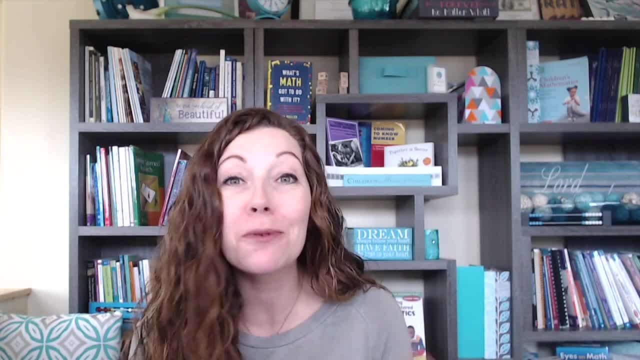 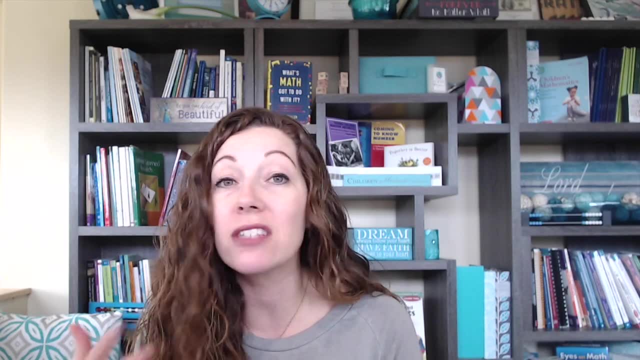 concrete, they have access to it. So we're doing a lesson that is concrete, and if some kids need the concrete, they have access to those manipulatives. if you're following rule number two, If kids don't and they just want to draw, then they can draw If they have moved past both of those and they're. 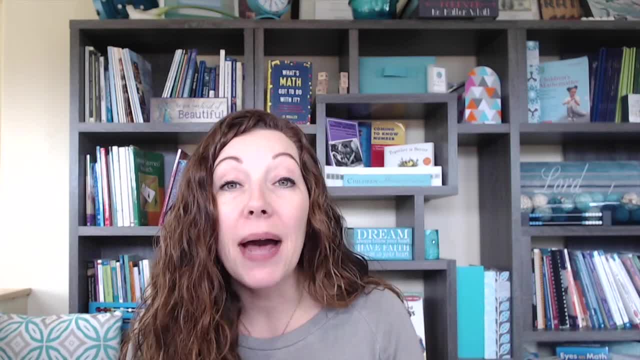 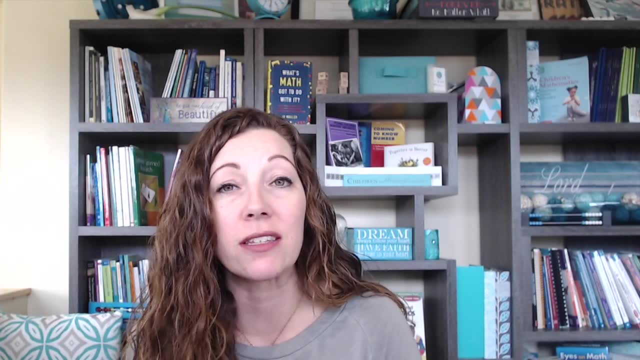 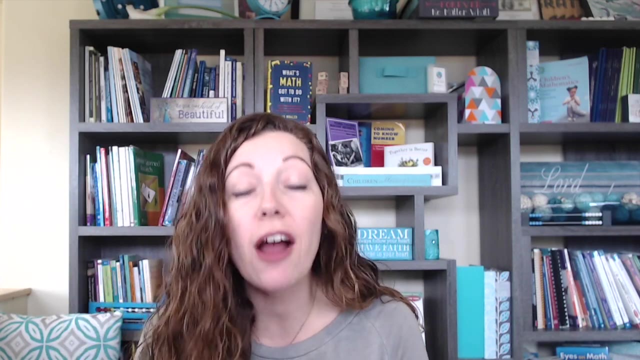 in the abstract world, then they're doing the abstract. But don't just do one of those. It's helpful for kids to be able to see all three and make connections. If the lesson says we're doing the concrete, it's fine Have kids model it, but be drawing a representation. Attach the abstract. 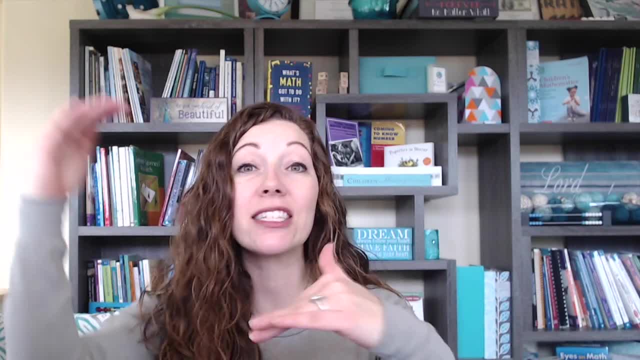 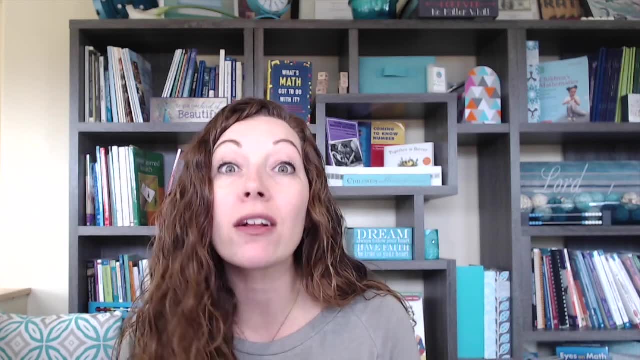 symbols to the abstract world. If you're doing the abstract world, then you're doing the abstract world to it as well, because you've got kids at all different levels And we talk so much about kids. we need to differentiate for all of our different learners, Yet our lessons don't often do that.